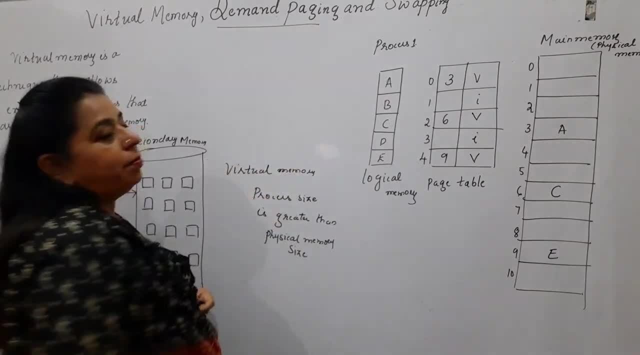 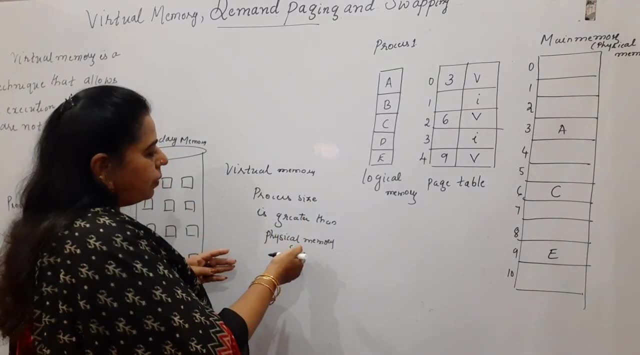 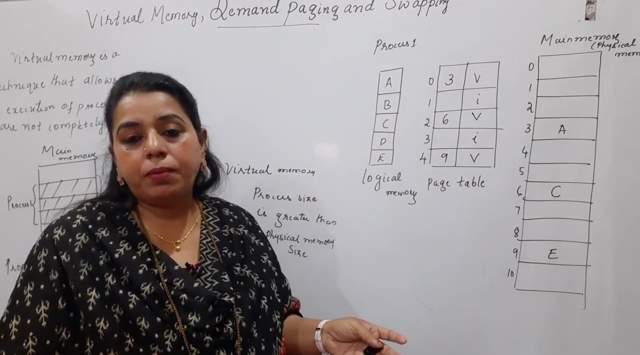 is it possible? it is possible with the help of demand paging, So virtual memory can be implemented using the demand paging. What exactly is happening in this concept is not all pages of the processes are loaded initially in the main memory. only on demand the pages are brought into the main. 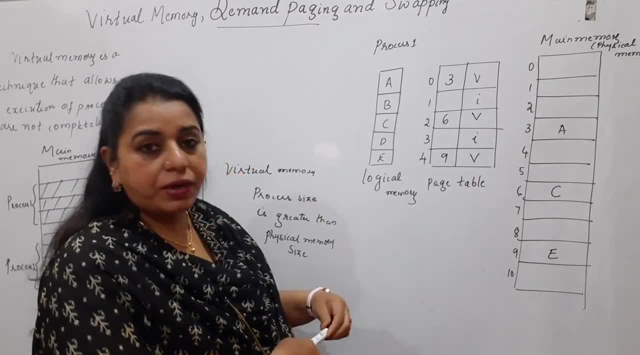 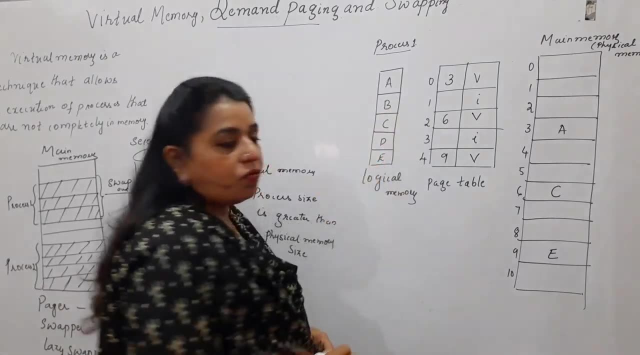 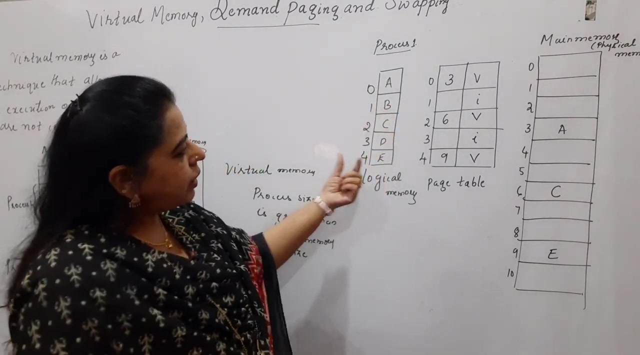 memory. so you can see, with this one example which i have written over here, look here, let us take: there is one process, p1. so here i am just writing. this process p1 has got some five pages, which are those a, b, c, d, e. so these are the five pages. now these pages are brought into the main memory only. 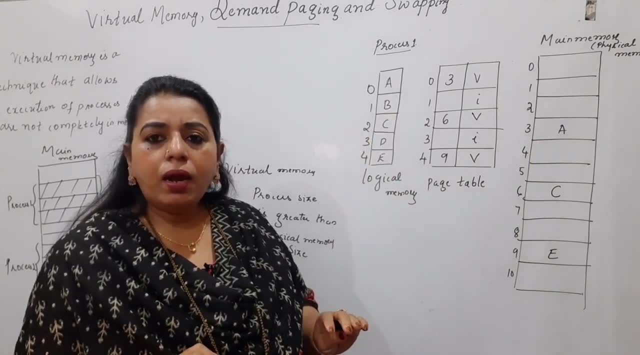 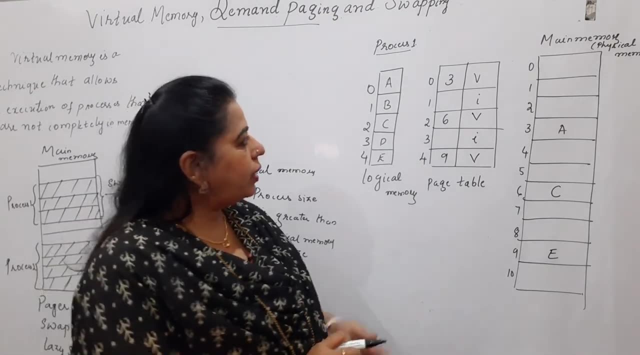 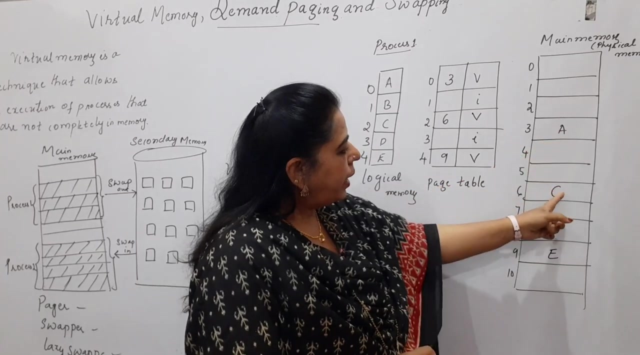 on demand. see, the reason is not all the pages will be used by the cpu at a time, only one after the other. the cpu tries to access the pages of a process. so here i have shown, out of the five pages, there are only three pages that are present in the main memory initially. so which are those pages? a, 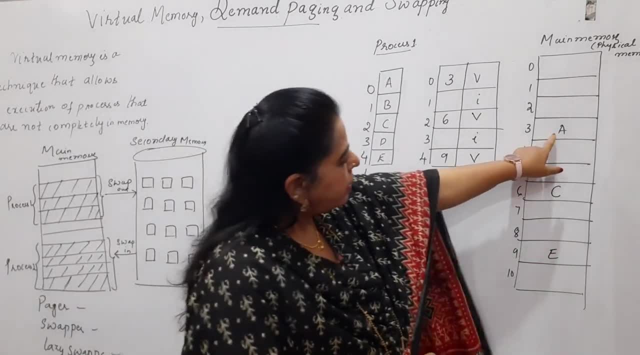 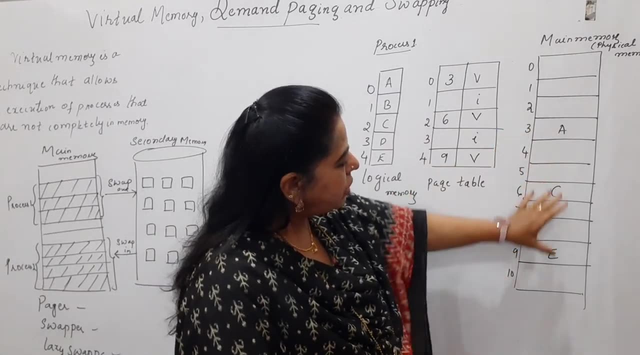 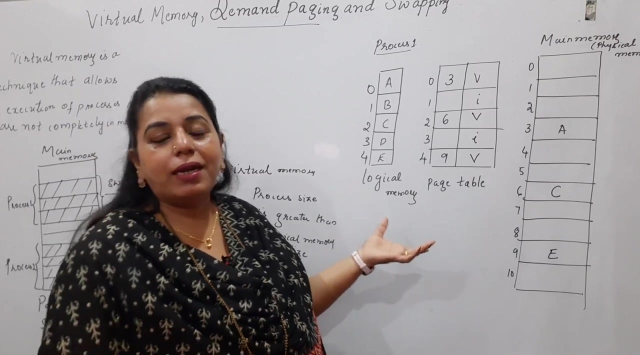 c and e. now what will happen? a is present in frame number three. c is present in frame number six. e is present in frame number nine. so only information about these three pages which are there, the physical memory, is shown in the page table. so you people are now completely aware what exactly. 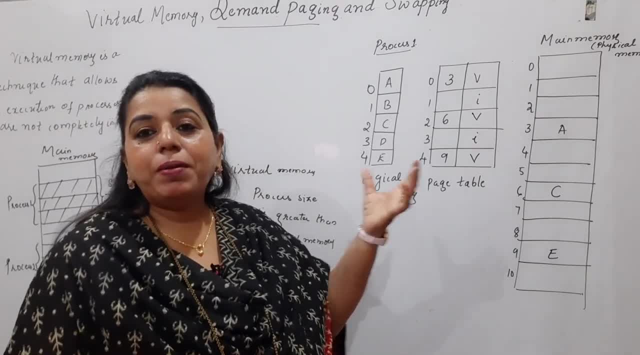 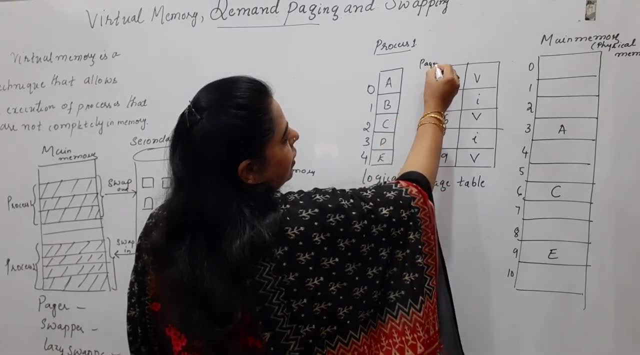 the page table holds. it holds the information about what, the frame numbers, where these pages are stored in the main memory. so you can check here. so these are the page numbers. what is that? indexing for a page table is always the page numbers and then you have the frame number and 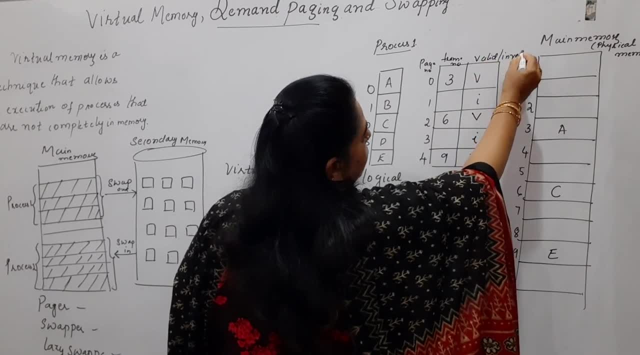 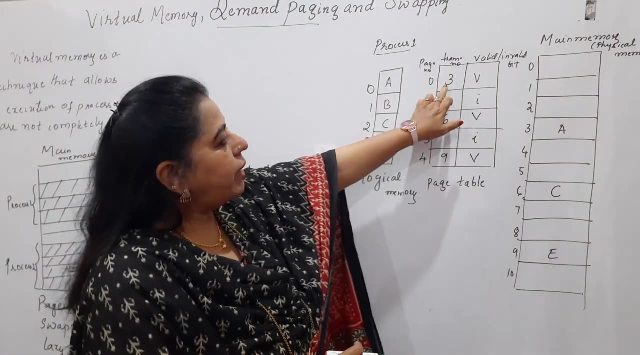 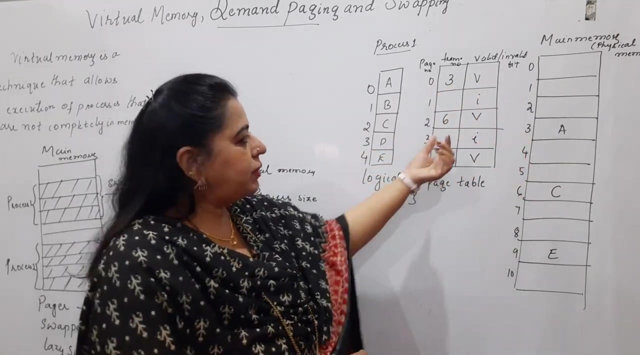 here you have another bit of information called as valid or invalid bit. what does valid and invalid bit indicates? valid bit indicates that the process page, the page of that particular process, is present in the physical memory. i indicates the page is not available in the physical memory. v indicates so this is what, since we have placed only three pages in the main memory and the frame. 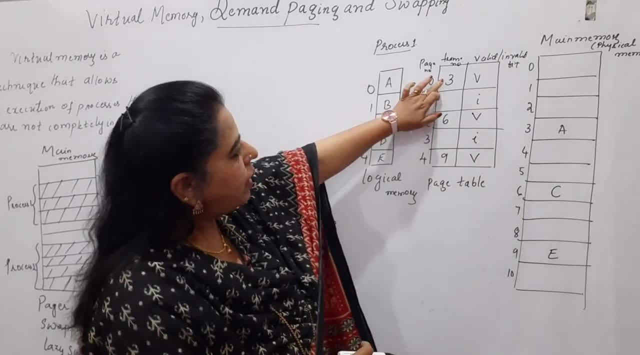 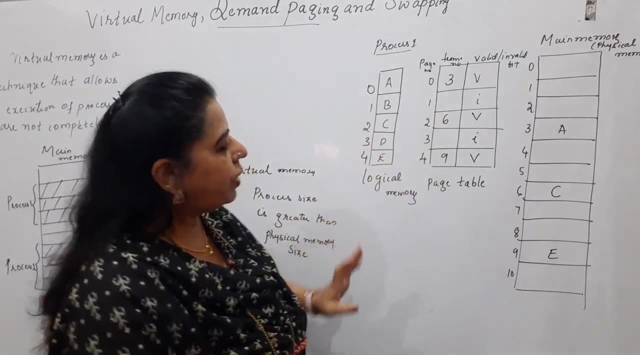 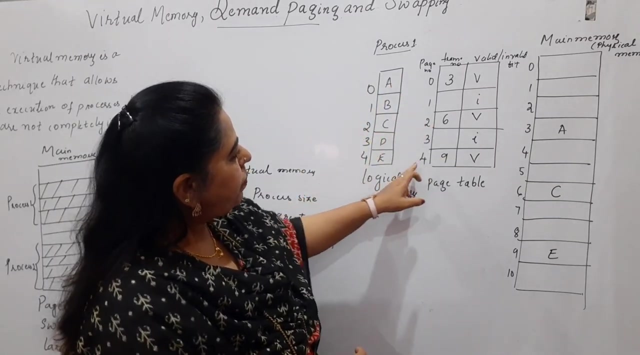 numbers are three, six and nine respectively. so you can see here: page zero is present in frame number three. page two is present in frame number six. page four is present in frame number nine. what is pay zero? page zero is a. what is page two? page two is C. what is page four, page? 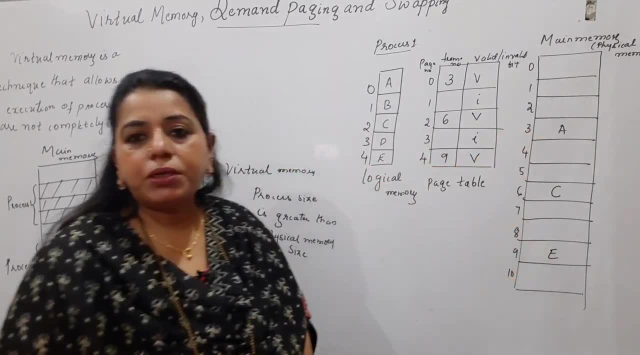 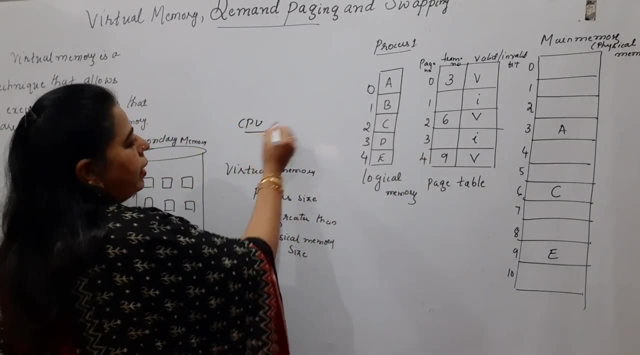 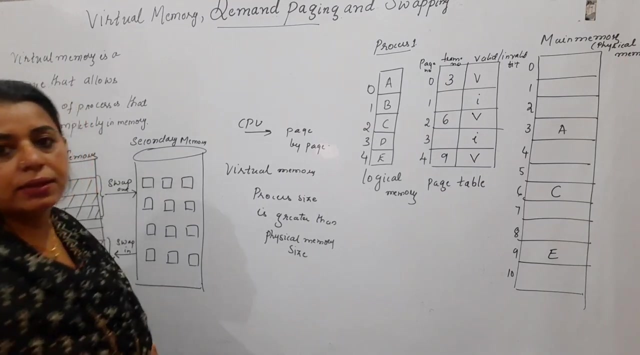 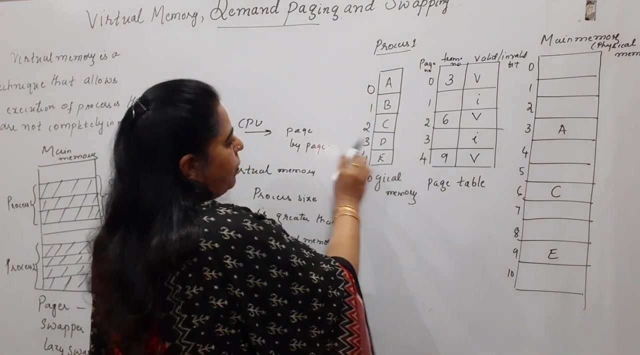 four is e. so a, C and e. the only information about these three pages are shown in the page table. so the CPU is always what? accessing the process, page by page, page by page. it is accessing the process, suppose, if I have to say that, yes, the process size is having five pages. okay, out of those five pages, the 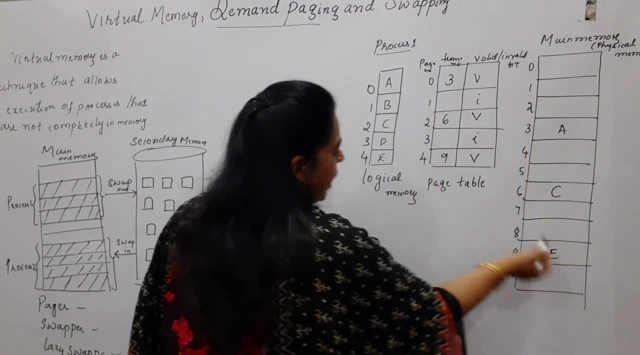 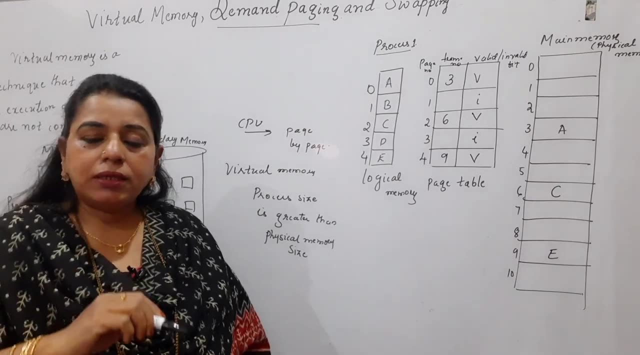 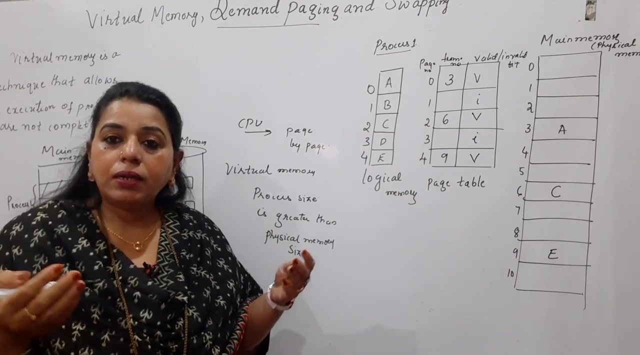 CPU is a trying to access only what page a? page C and page e. so only those pages will be brought into the main memory. on demand the pages are brought into the main memory. that's why we say: demand paging. only on demand you bring the pages into the main memory. in this way only we can afford the complete pages of. 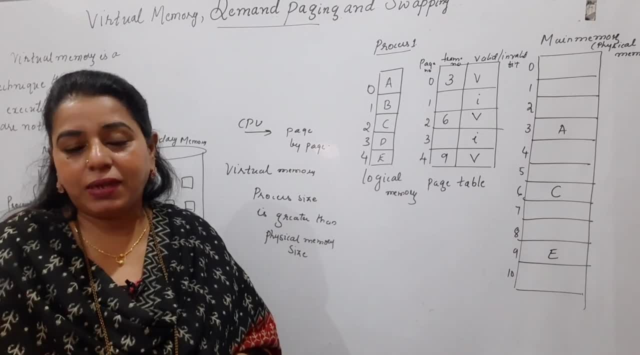 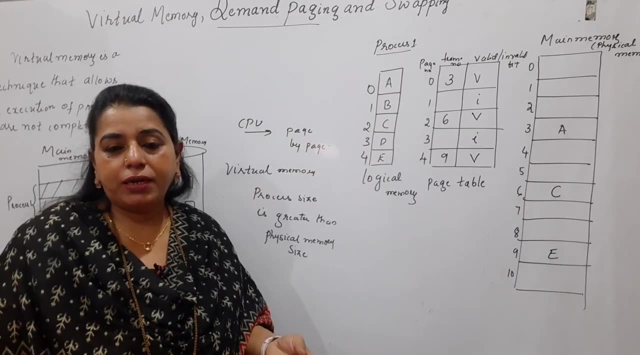 a particular process whose size is larger than the size of the physical memory, for example. if you say that you want to see even at present- nowadays we also have laptops with what physical memory, that is, the RAM capacity, as 4gb, 8gb. earlier we were having just with the 2gb. 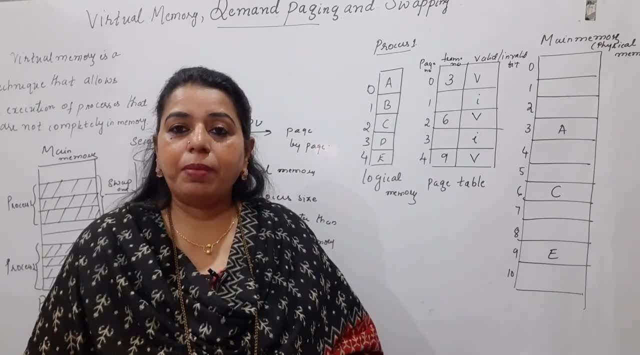 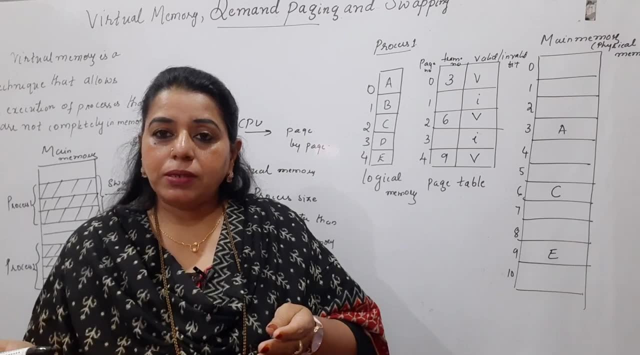 RAM. but when we were watching a movie, which is suppose, if your RAM capacity is 2gb and you are watching a movie of 6gb, how is it possible that? that is why that is possible, because the initial part of the movie which is first loaded into the 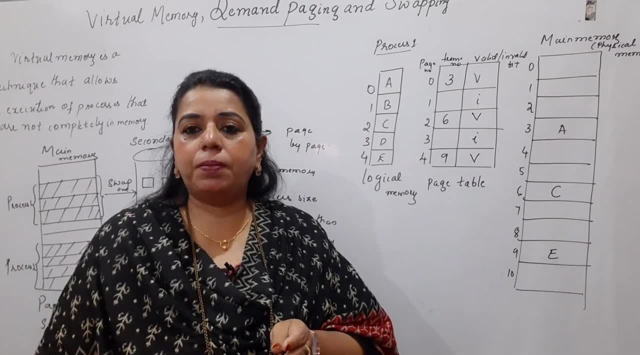 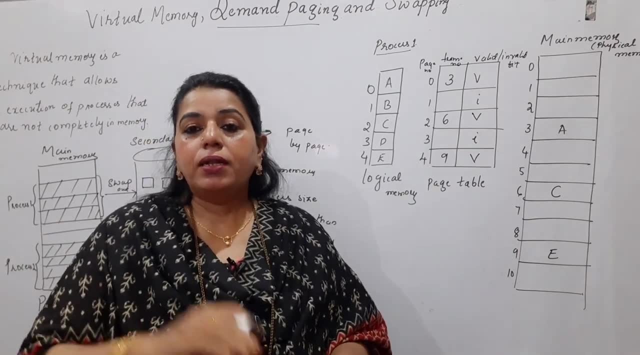 main memory. so suppose if your RAM capacity is 2gb, only the first part of the movie. let us take, for example, the first 15 minutes of the movie is more loaded into the main memory. next 15 minutes gets loaded into the memory. when the memory capacity becomes full, then the first 15. 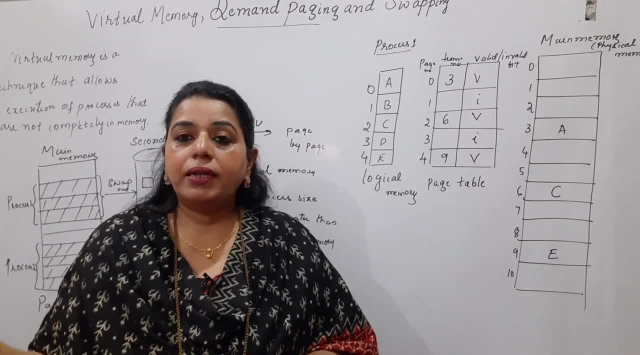 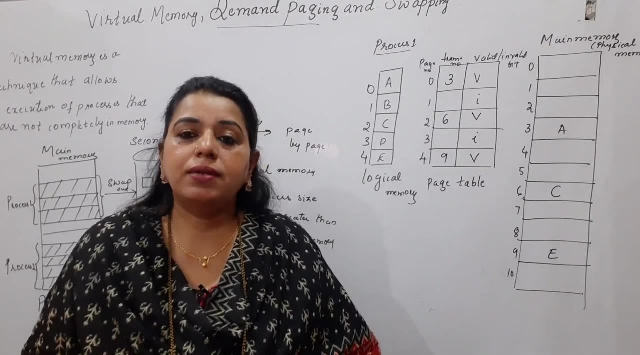 minutes that were initially loaded will be brought out from the memory, and then the next 15 minutes of movie will be loaded into the main memory. this is how, though, your physical memory size is lesser than the size of the movie, but still you are able to watch the complete movie. so that is what is what demand. 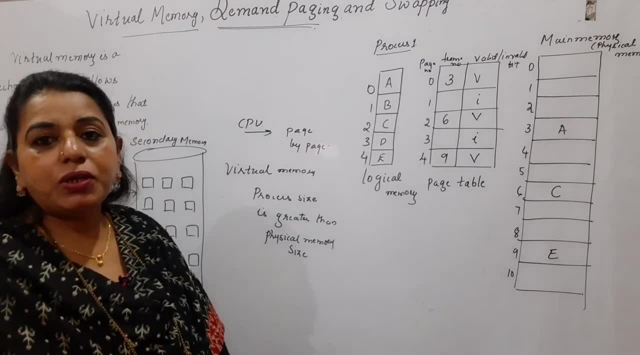 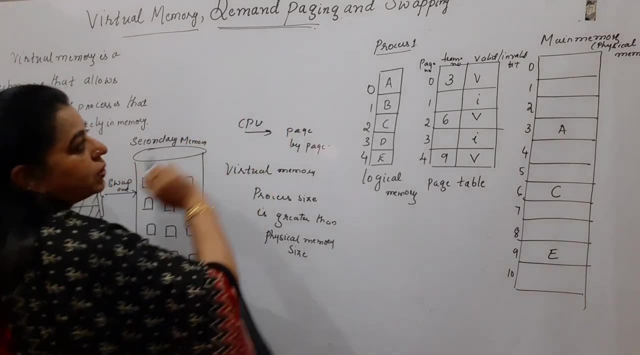 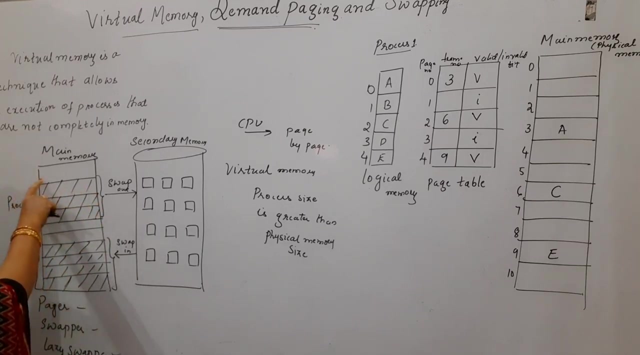 paging and we say that memory as virtual memory. that is not real. look here and also you should know this concept: swapping is also interrelated with this virtual memory. only you can see here, this is the physical memory. one example I am just giving: there is one process called process 1. process 1 is having 3. 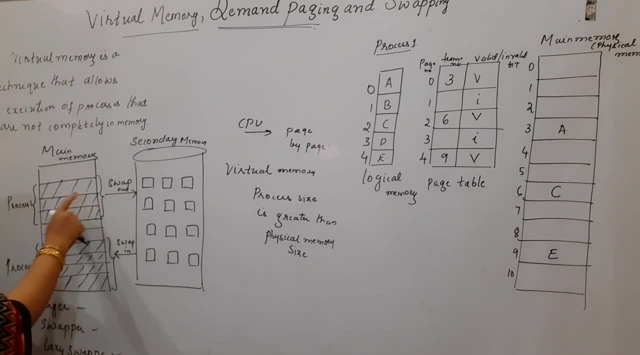 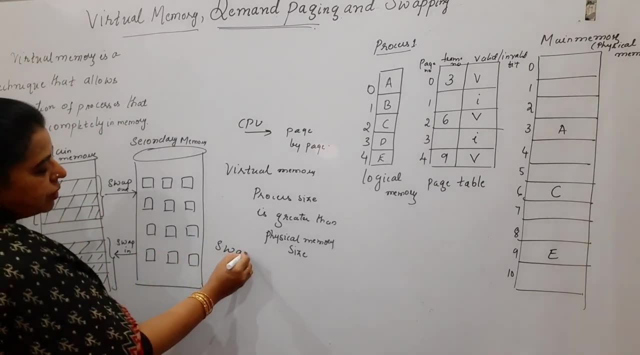 pages. process 2 is having 4 pages. any point of time, if at all any other process has to be brought into the memory, is swapping takes place. so there is a module called which will swap out the pages of the process. Now, here in this swapper is a one which is going to: 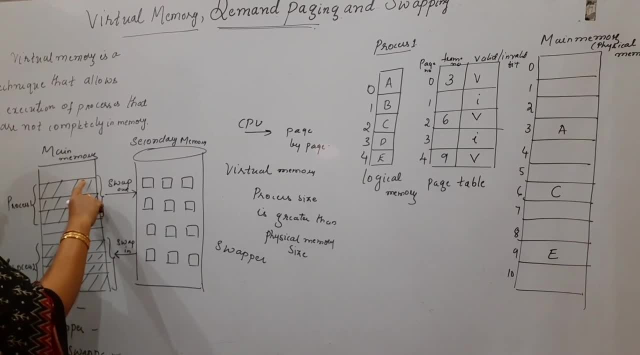 swap the entire process. That means if there are three pages belonging to the process, all the three pages are brought into the secondary memory. Swap in is bringing the pages from the secondary memory to the main memory. Now, here also, when you are swapping in, you are bringing all the pages of. 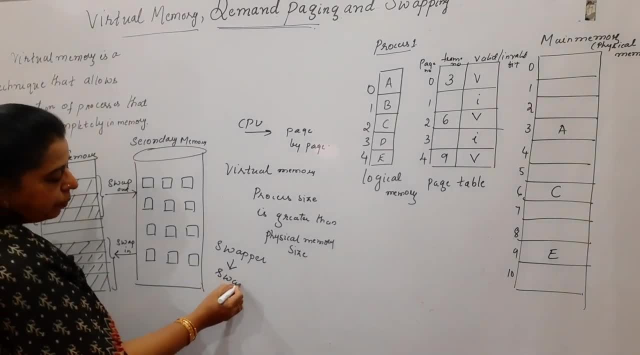 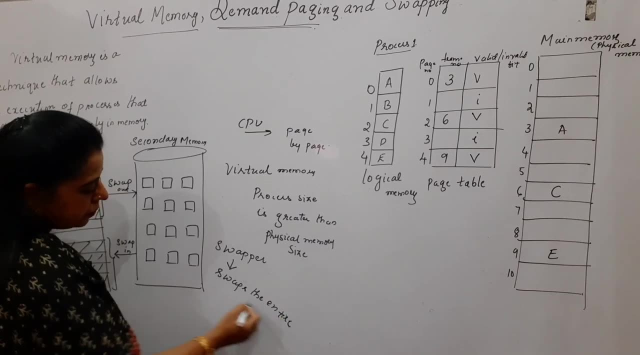 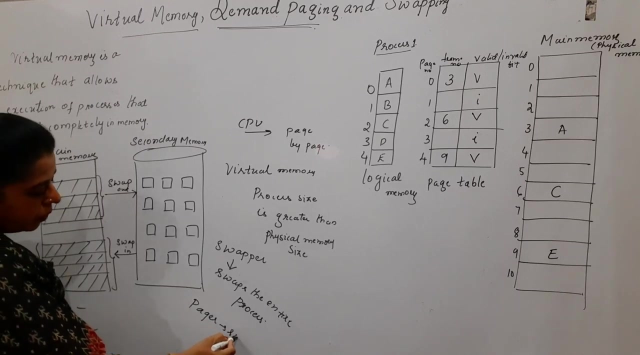 that process. So swapper always what swaps the entire process. Remember the difference between swapper and pager. Swapper swaps the entire process, whereas pager will swap only a particular page. Swaps the page of a process. Page of a process Only on demand, if the page has to be. 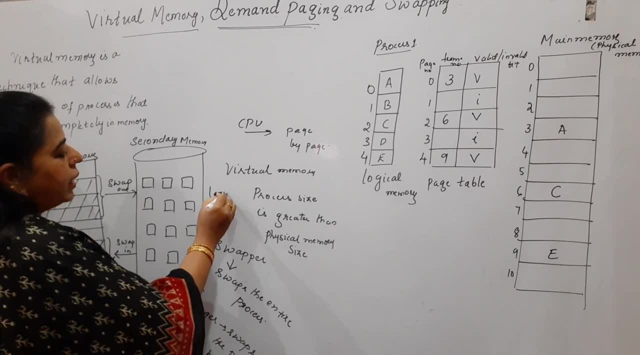 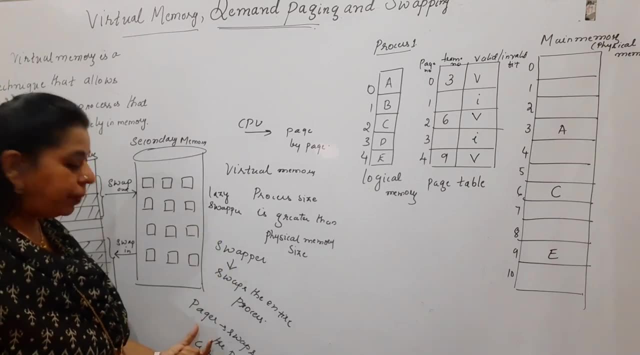 brought into the main memory. then we say the module which is carrying out this task as lazy swapper. So hope you people are getting the difference between all these three terms: swapper, lazy swapper and pager. So in continuation with the demand paging, there is also one more term. 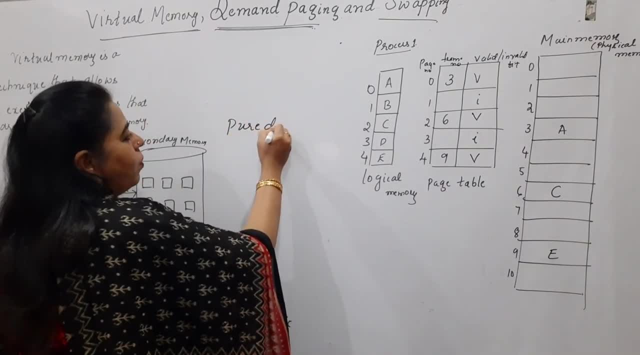 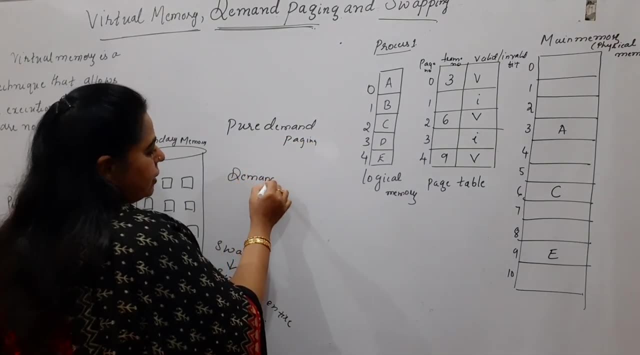 associated with it. It is called as pure demand paging. Now, what is the difference between demand paging and pure demand paging? First, let me tell you about the demand paging. Demand paging, as I said just in the beginning of my session, this session, once again with an example. I will try. 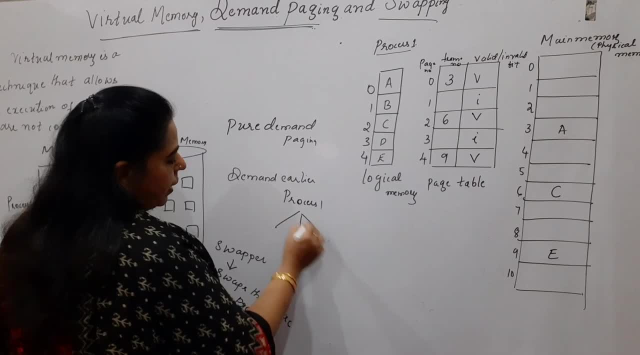 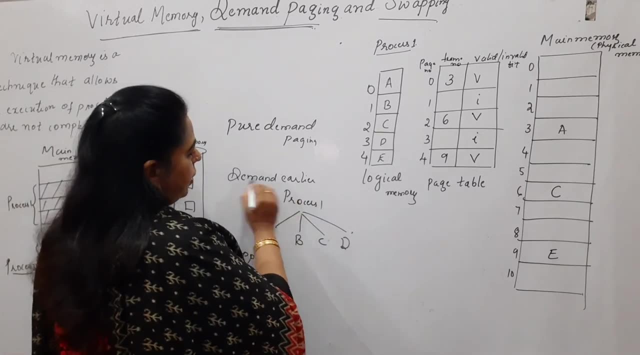 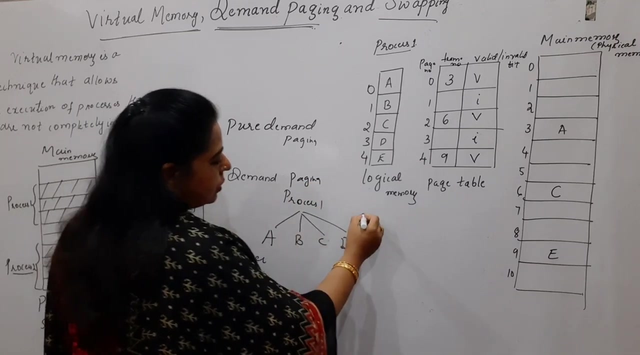 to tell you there is one process. let us assume process one. Process one has got four pages. Let us assume four pages are there belonging to process one. So in demand paging, what exactly is happening is? let us first assume that out of all these four pages, of process one, 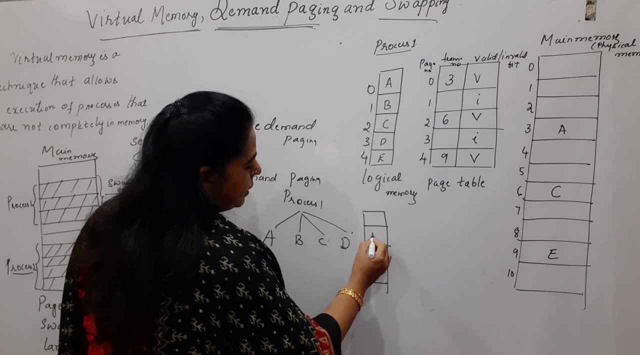 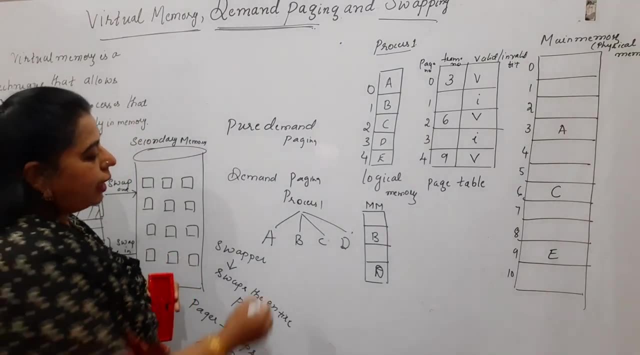 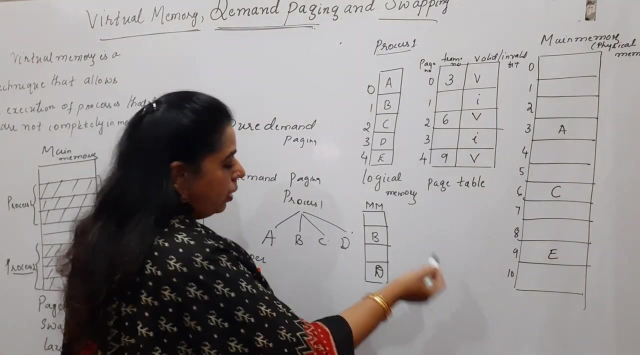 in the physical memory there are only two pages that are present: b and c. b and d. Let us assume b and d are present in the physical memory or the main memory. Now the CPU wants to execute an instruction belonging to page c. Page c is not present in the main memory. Then it will be. 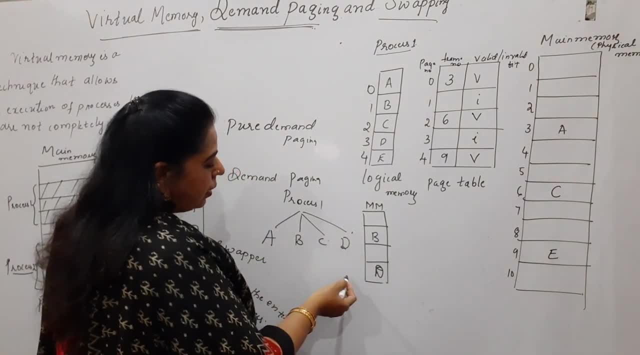 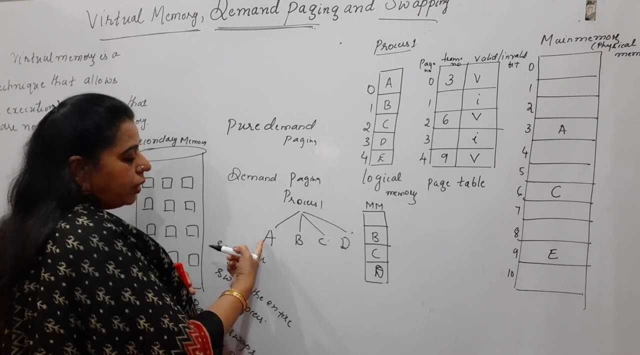 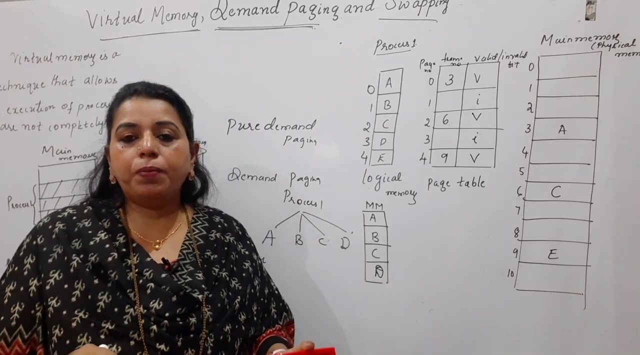 brought into the main memory on demand. So we say that there is a demand paging happening, So c will be brought into the main memory. Similarly, next time CPU wants to execute an instruction belonging to page a, then page a will be brought into the main memory. So in demand paging initially few. 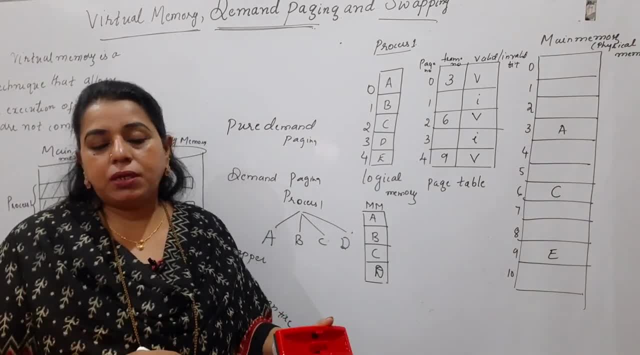 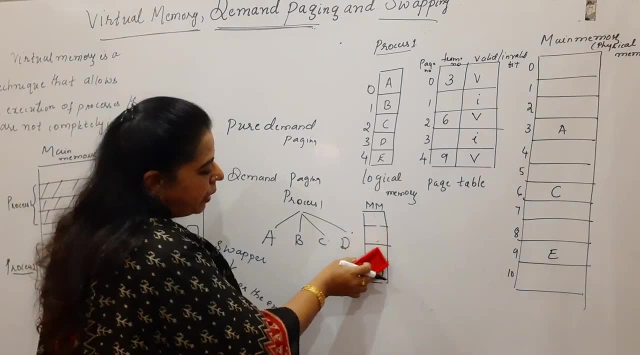 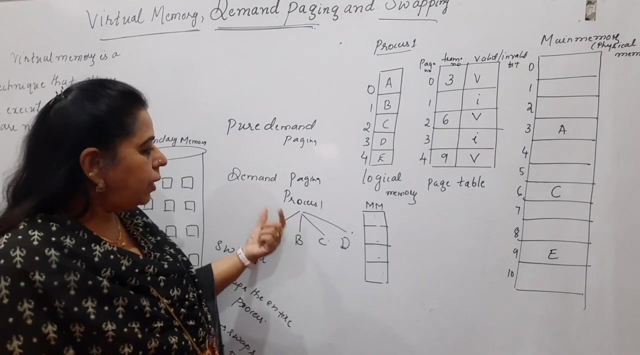 pages were already there in the main memory. Few pages which the CPU wants to access were brought into the main memory, But in pure demand paging. not a single page of that process is present in the main memory. You can see here: all these four frames of the main memory are empty. The CPU has 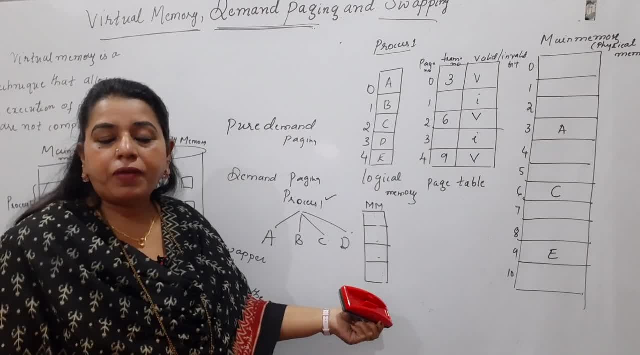 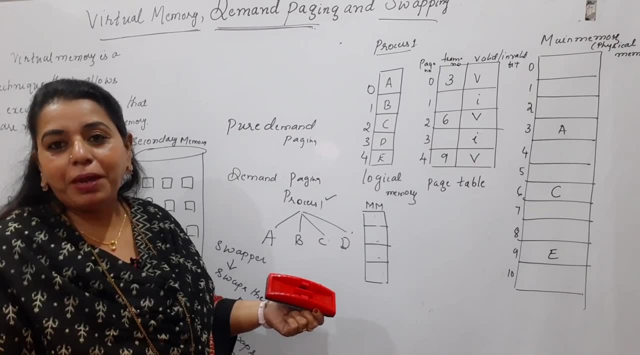 started executing what the process p1.. So that means now CPU is not finding any page of that process present in the main memory. So now, one by one, all the pages has to be brought into the main memory. So that is how we say when the complete main memory, that is all the frames, are empty and 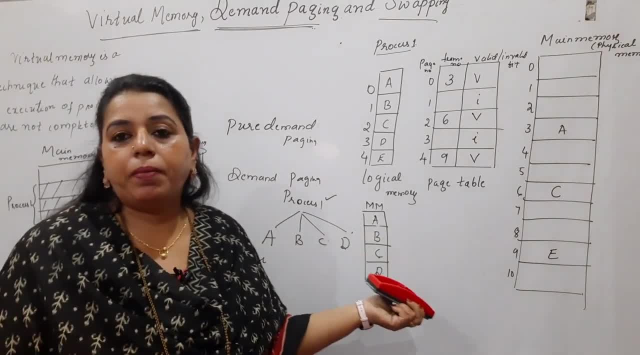 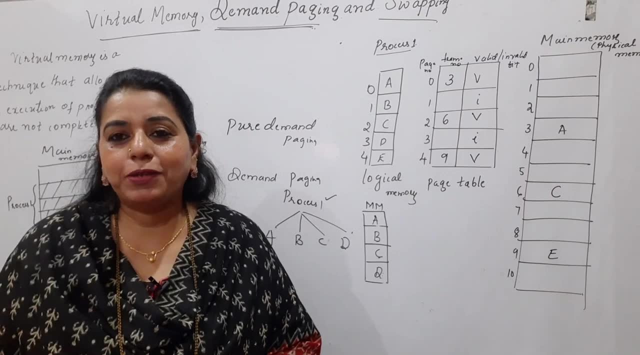 then, on demand, one by one, all the pages get in inside this main memory or get placed inside this main memory. We say this type of concept as pure demand paging. Not a single page of that process was present in the main memory. Moreover, from where these pages are getting loaded into the main memory, it is from 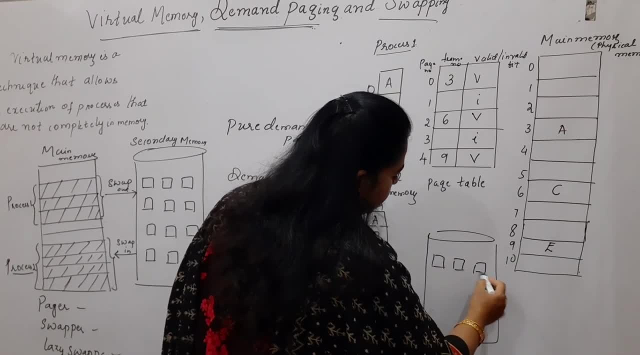 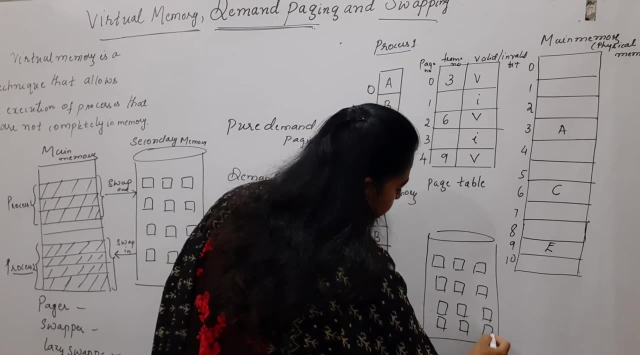 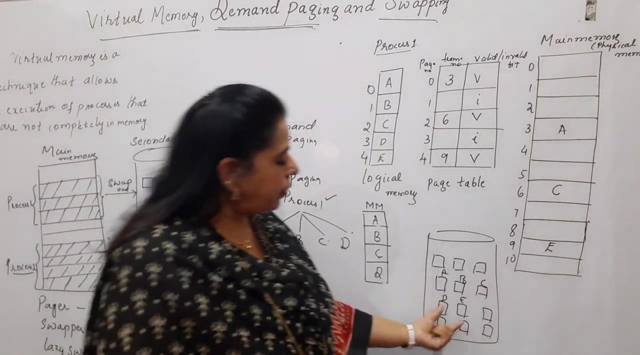 the secondary memory. So if you are having what number of pages, I can show it with this diagram in the secondary memory. So out of how many All pages are what present in the main memory? only Let me show it here. a, b, c, d and e, These five pages belong to process p1. So from here these 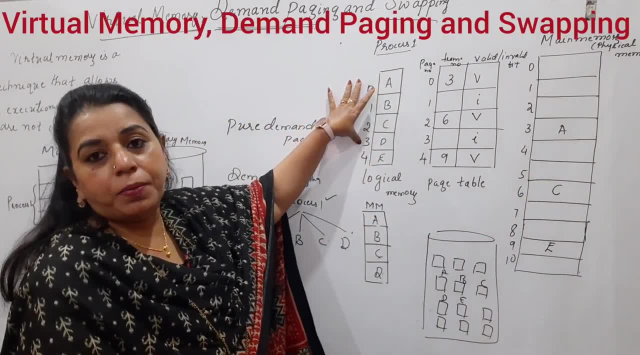 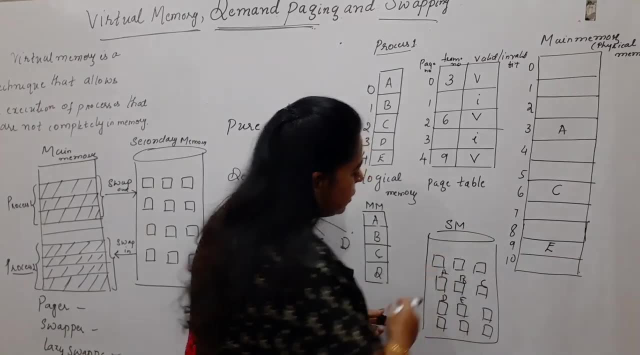 pages are loaded into the main memory, But what I am showing here in this is what The virtual memory. So this virtual memory can be shown with a diagram in this manner, Whereas for the secondary memory, which is hard disk, you are showing all the pages of that process in this manner, And whereas for 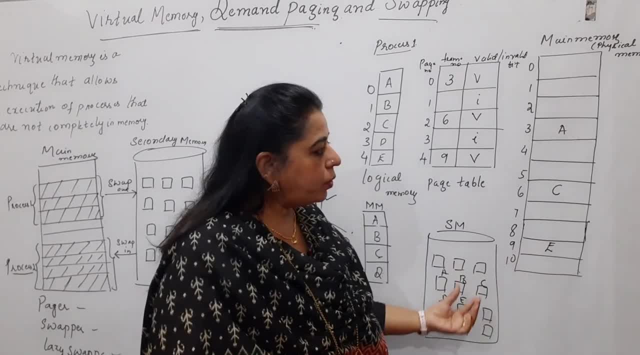 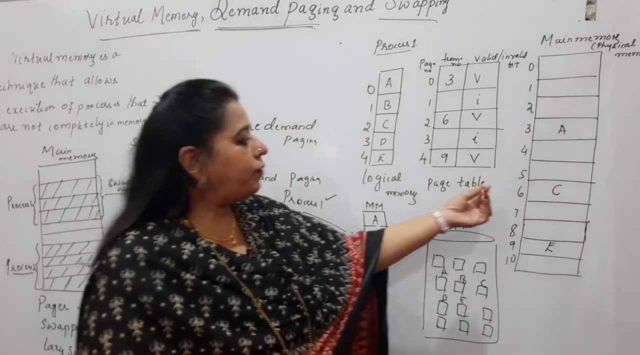 the main memory. you can represent it in this diagram And also, moreover, you have to show that how many pages and which pages of that process p1 are loaded into the main memory. And apart from that, you have to show that in the page table in which frames of these physical memory 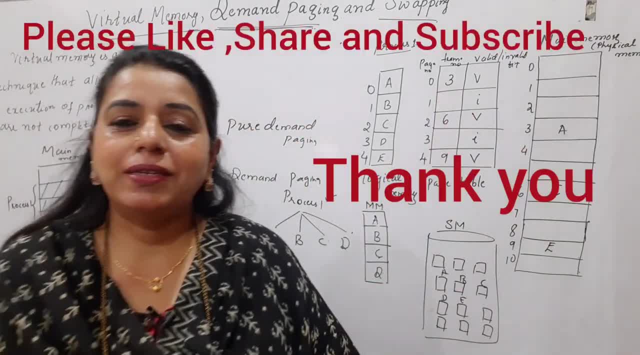 are the pages of those processes shown. Hope you find this session useful. Please like, share and subscribe to my channel. Thank you, Bye, bye, Take care.